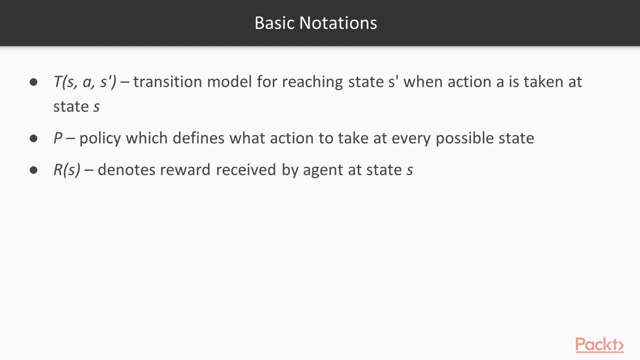 The basic motivations for RL are shown. T of S A S bar represents the transition model for searching state S bar when action A is taken at state S Next. P represents a policy which defines what action to take at every possible state. R of S denotes the reward. 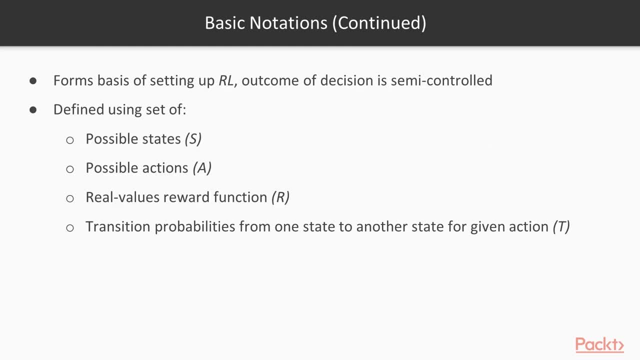 received by agent at state S. The Markov Decision Process forms the base of setting up RL, where the outcome of a decision is semi-controlled, that is, it is partially random and partially controlled by the decision maker. An MDP is defined using a set of possible. 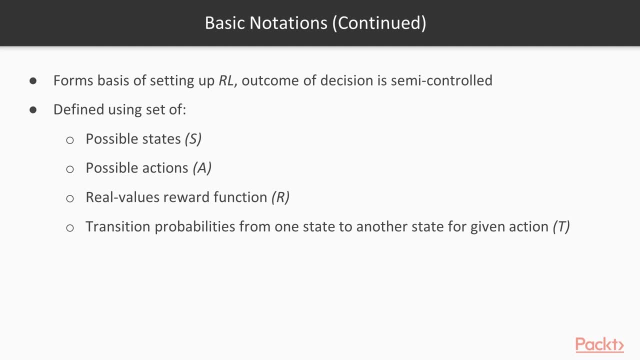 states S as set of possible actions A, a real values, reward function R and a set of transition probabilities from one state to another for a given action T. In addition, the effects of an action performed on one state depends only on that state and. 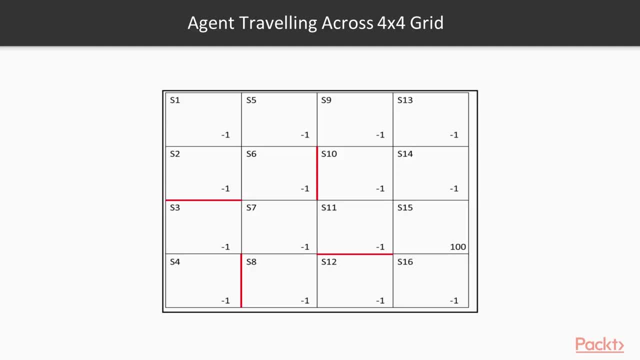 not on its previous states. Now let us define an agent traveling across a four-by-four grid. as shown here in this figure, This grid has 16 states. In each state, the agent can perform four actions: up, right, down and left. However, the agent will be. 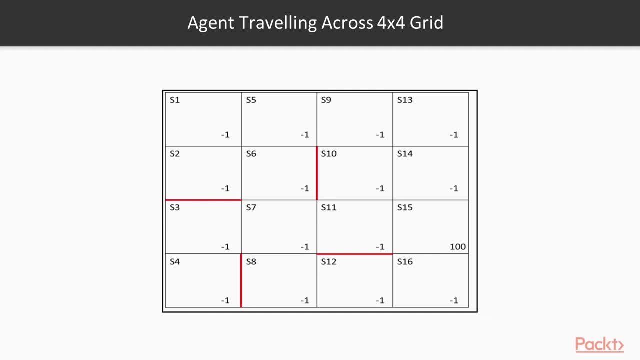 restricted to some actions based on these constraints, The states across the edges shall be restricted to actions which point only toward states in the grid. For example, an agent in S1 is restricted to the right or down action. Some state transitions have barriers. 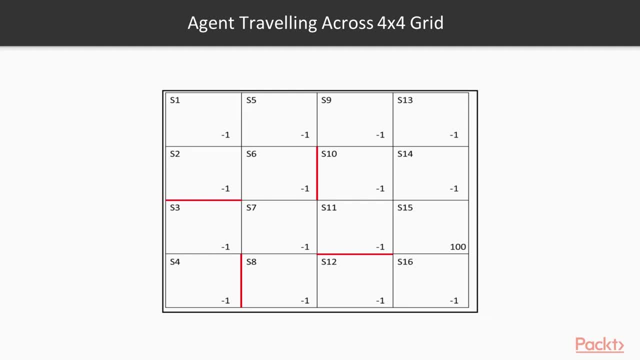 marked in red. For example, the agent cannot go down from S2 to S3.. Each state is also assigned to a reward. The objective of the agent is to reach the destination with minimum moves, thereby achieving the maximum reward. Accept state S15 with a reward value of 100.. All the remaining states have a reward value. 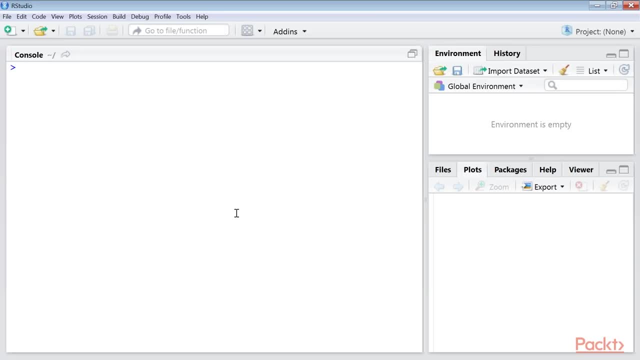 of negative 1.. Now we will see how to set up RL models using MDPToolBox in R. First, install and load the required package. Define the transition probabilities for action. Here each row denotes from state and each column denotes to state. As we have 16 state models, the change would also be gentle In. 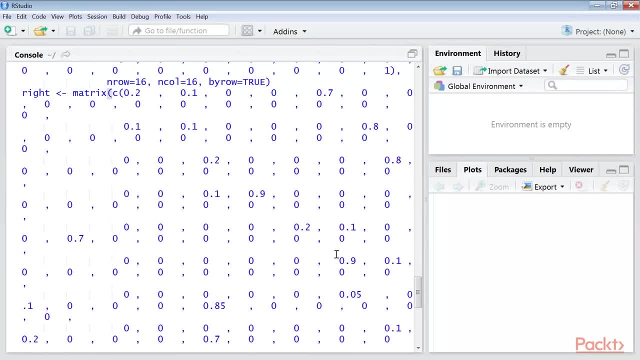 this case, each column denotes to state and each column denotes to action as well. as we have 16 states, So we can define the transition probabilities for action, Our action would be. the transition probability matrix of each action shall be a 16x16 matrix, with each row adding up to 1..